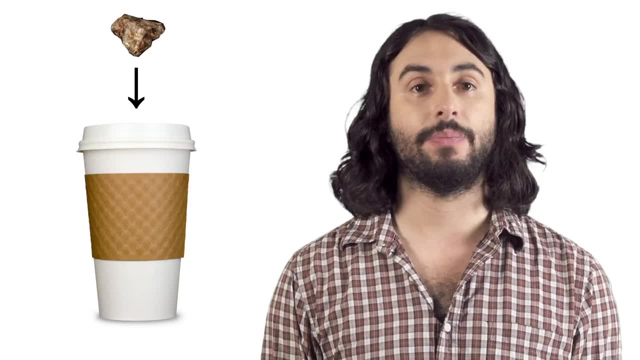 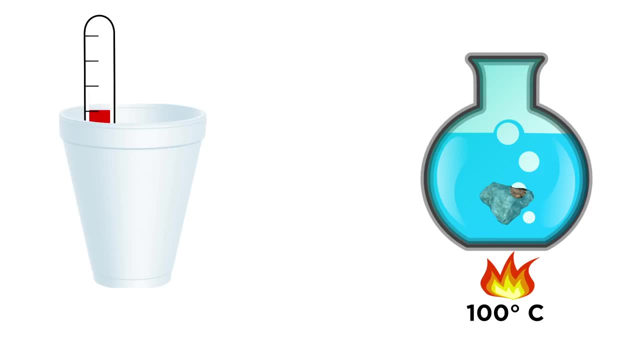 information to calculate the specific heat of the metal. so let's say you heat up a metal by placing it in boiling water at a known temperature until it is just as hot as the water. then, with tongs, you place it in a coffee cup. 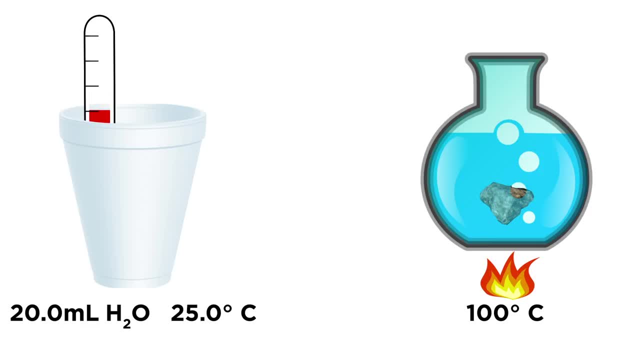 containing a known volume of room temperature water. with a thermometer, the water in the cup will heat up slightly as the heat from the metal flows into the water, and we can record the resulting temperature change from there. we just do some math. we use the specific heat equation. 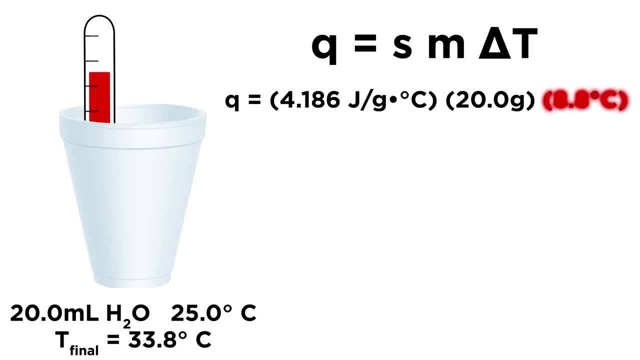 and plug in the data. for the water, the temperature change is what you recorded. the mass of water in grams is equal to the number of milliliters of water. the temperature change is what you recorded. the heat from the metal is equal to the number of milliliters of water and the specific heat of water. 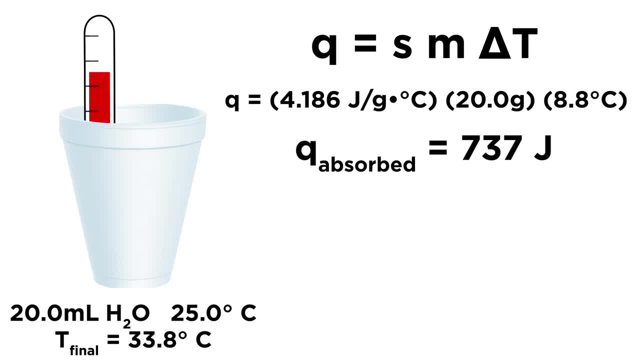 is a known value. this allows us to calculate the heat absorbed by the water. well, the heat absorbed by the water was the heat released by the metal. so we can take that same quantity of heat and plug it into a new equation for the metal. that value goes there. we weighed the metal beforehand. 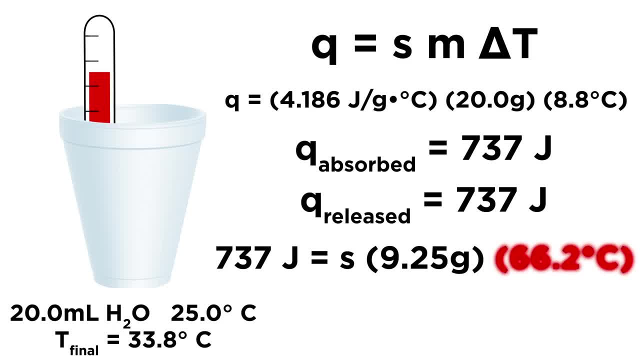 and this time the temperature change of the metal is from the boiling water to the final temperature in the coffee cup, so you can solve for the specific heat of the metal. this is useful for identifying unknown metals if you are given a few different specific heats. 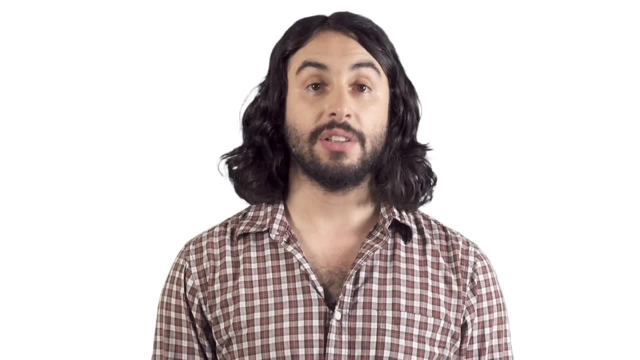 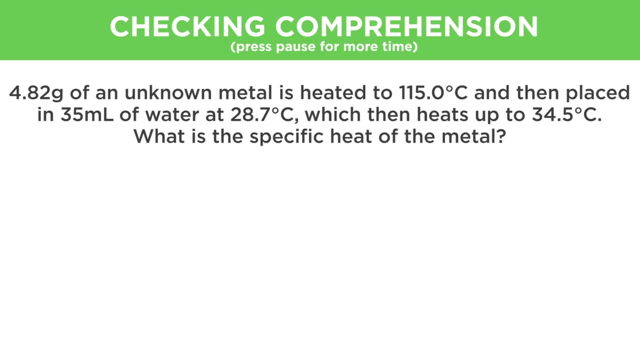 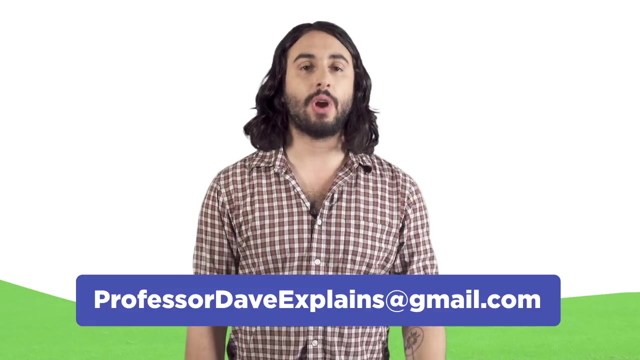 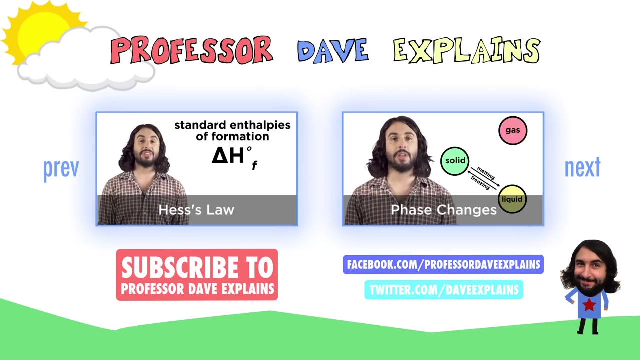 and asked to decipher which metal you are given. let's check comprehension. thanks for watching, guys. subscribe to my channel for more tutorials and, as always, feel free to email me professordaveexplains at gmailcom. I'll see you next time.